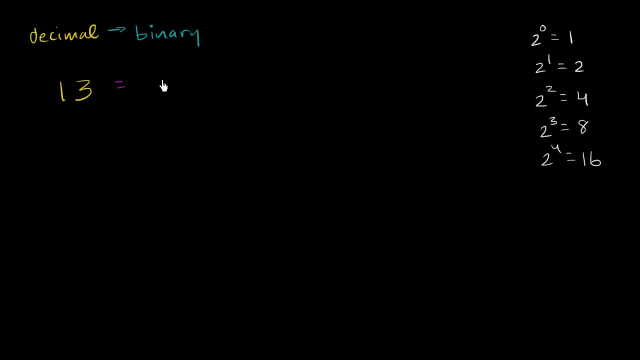 Well, 16 is too large. Well, it would be 8.. So I could rewrite 13 as 8 plus 5.. Now, 5 is not a power of 2, so I have to keep deconstructing that. 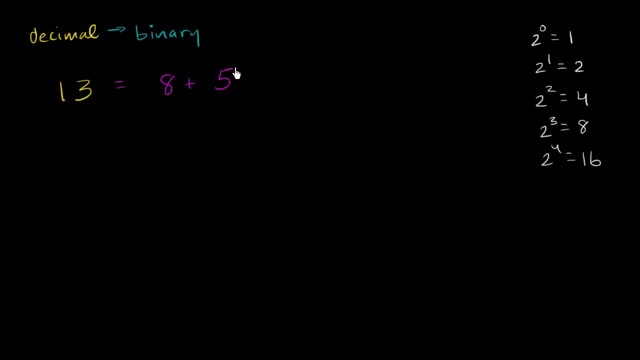 What's the largest power of 2 that is less than or equal to 5?? We see it right over here: It's 4.. So let me rewrite that It's 8 plus instead of writing 5,, I'll write 4 plus 1.. 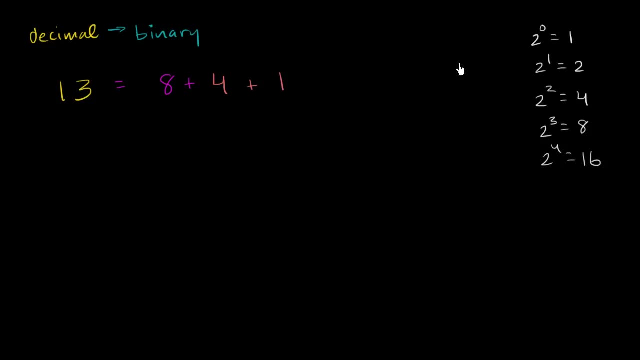 And then the good thing is: 1 as a power of 2, we already see the largest power of 2, that's less than or equal to it, is 1.. This already is a power of 2.. So I've now rewritten this as the sum of powers of 2.. 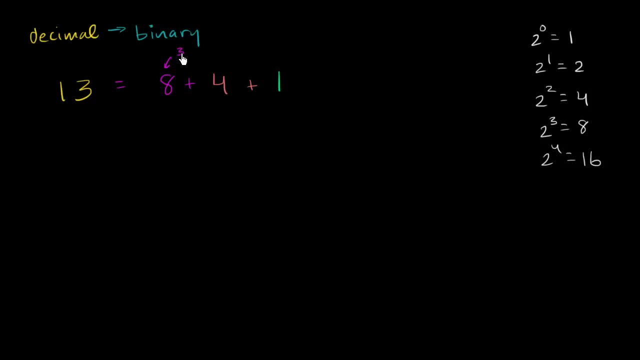 Notice: this is 2 to the 3rd Whoops, This is 2 to the 3rd power, This is 2 squared And this is 2 to the 0 power, Or I could write it like this: I have 1, 8.. 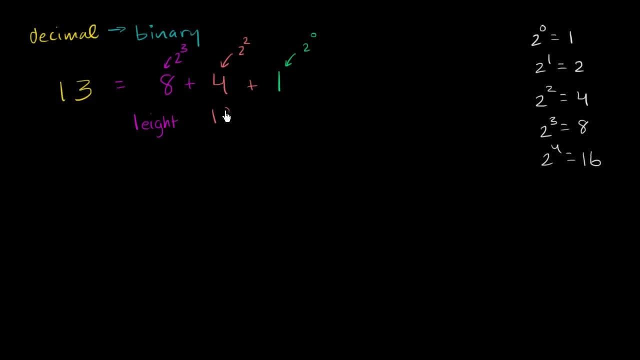 I have 1, 8,. clearly, I have 1, 4.. 1, 4.. Or, and I should say and, and I have 1, 1.. So I could add these two, I could add these three together. 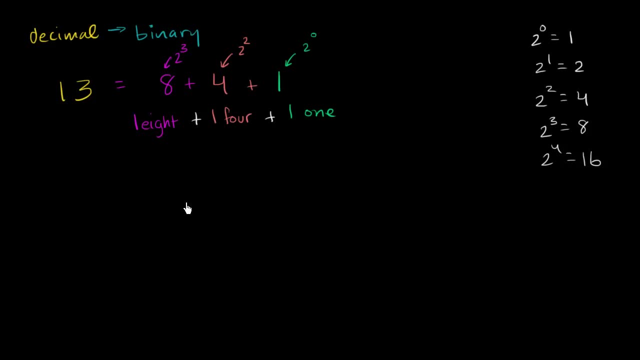 13 could be considered 1, 8 plus 1, 4 plus 1, 1.. Well, why is that helpful? Well, now let's go into binary mode and think about what each of the place values represent. So this is the 1's place. 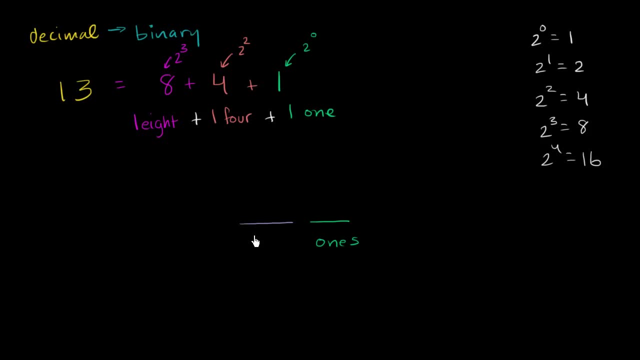 That's the 1's place, And then we could go to the 2's place, 2's place. Every time we go to the left, each place, we multiply by 2.. It's the next power of 2.. Then we go to the 4's place. 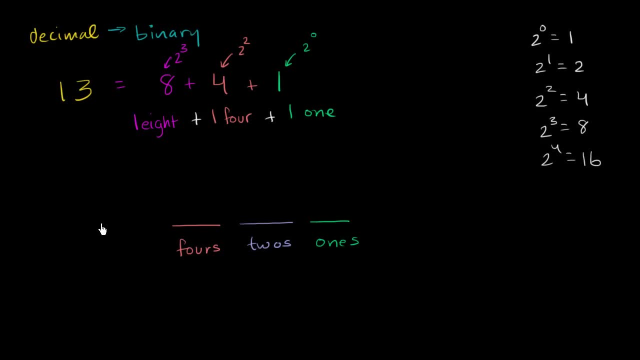 4's place, And then we go to the 8's place, 8's place, 8's, And in binary I only have two digits: 0 or 1.. So I either have 0 of a place or I have 1 of it.